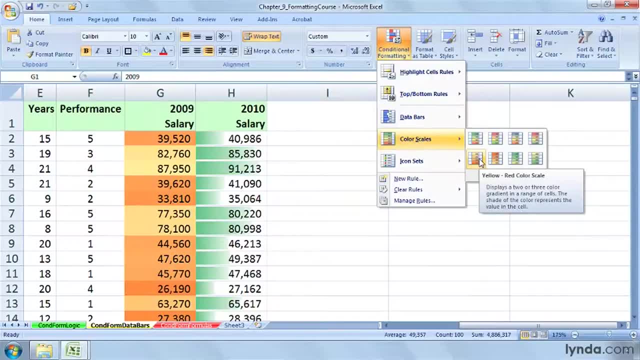 the data based on percentages And in fact, it's analyzing all the data in column G, dividing it into fifths and applying different colors based on that. you ultimately have the ability to change that. let's say, for the moment we'll just pick one of these and leave it that way. 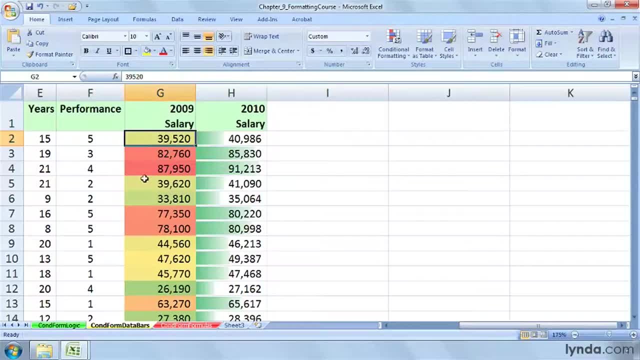 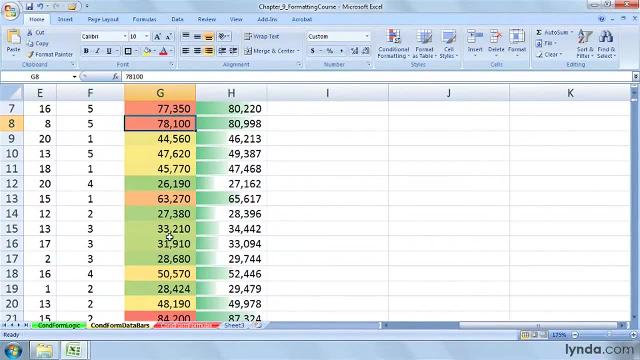 but you get the general idea here in looking at the salaries here in this example the higher salaries are reddish, those not quite so high, or well, those are pretty high there, but you see what's happening. here's one that's not quite as high, that's sort of an orange, and you see the other. 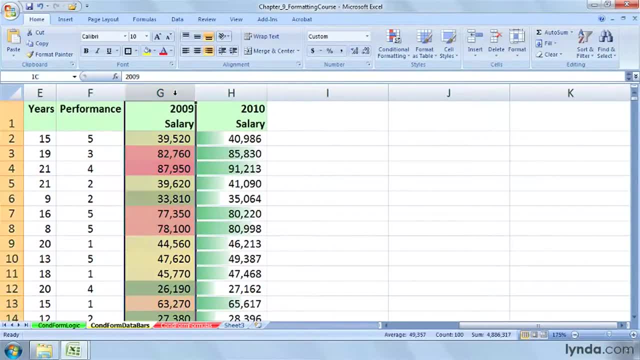 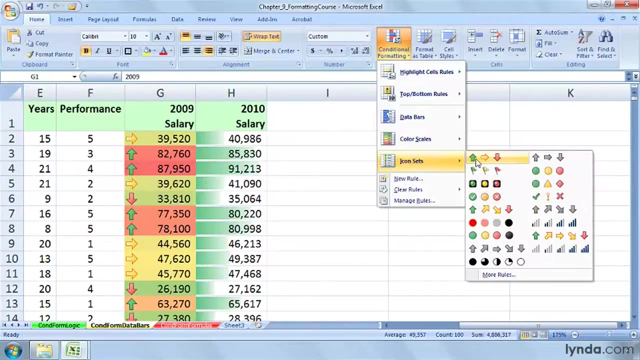 color variations taking place there. now, working on column g, again, let's go back to conditional formatting and also recognize that in addition to data bars and color scales, we also have icon sets, and i didn't remove the color, so possibly you might want to include a combination of these. 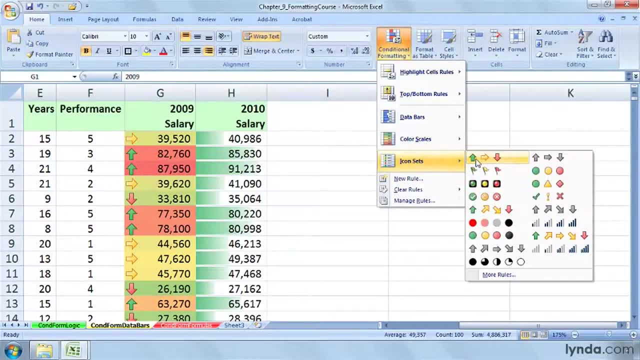 i think that's overkill myself, but we could do this and looking at this effect that we're about to see, you decide: well, that's too much going on there. what might we do here? click back on color variations and we can see that we have a lot of color variations taking place there, so 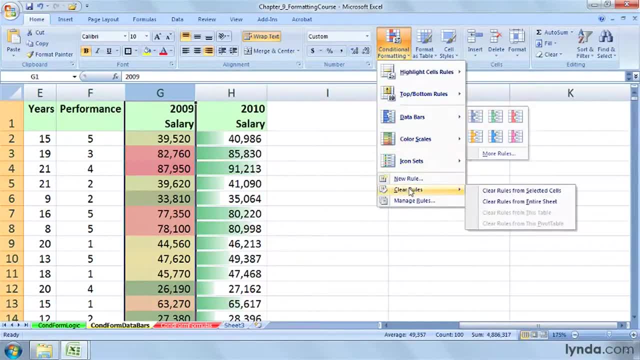 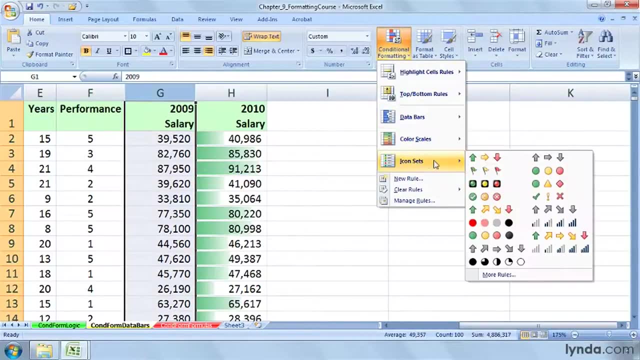 click back on color variations and we can see that we have a lot of color variations taking place. conditional formatting and choose clear rules from selected cells. now let's try conditional formatting icon sets and we see some of these choices i think you can see here. it's going to take you a while to decide which one you like, although here and there one's. 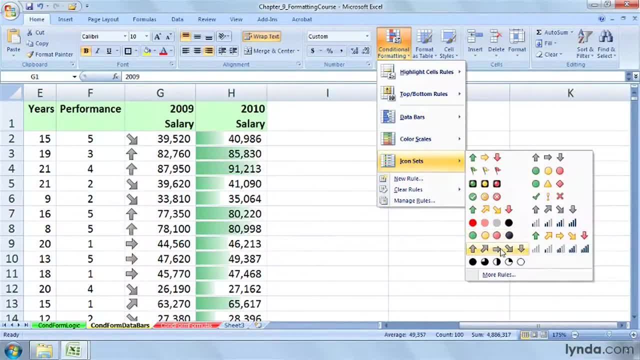 going to jump right out at you. if, for example, i were to choose this one here with the different gray colored arrows, you'll recognize that the arrows that point upward are the higher salaries, those that point downward are the lowers and those that point down are the lower salaries. 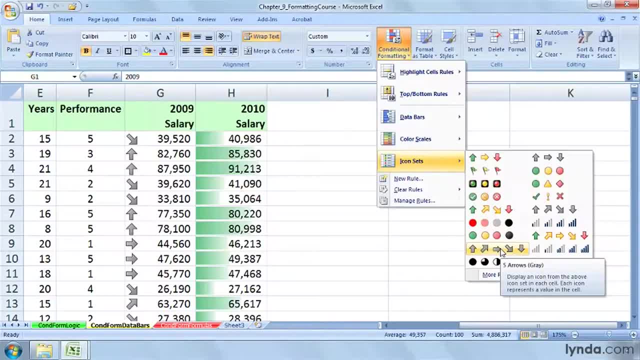 other arrows point rightward, or you might say northeast or upper right, southeast, lower right, and so on. you see what's happening here too. the data is divided into, in this case, fifths or percentiles, 20 percentiles. so you have a favorite here or there. maybe we'll choose this one. this is: 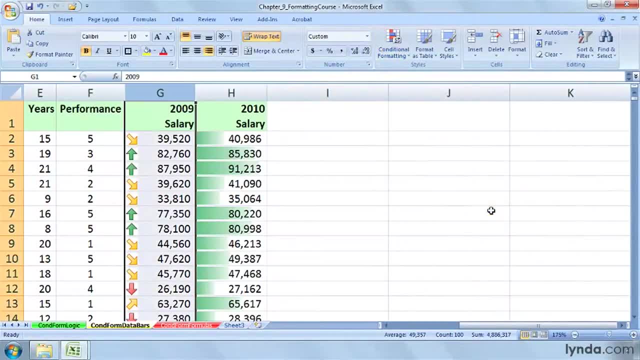 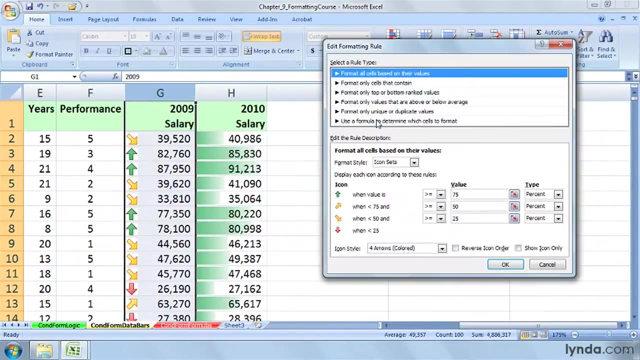 dividing the data into quarters, and maybe that's just what you want. but if you want to fine-tune this- and you can- you can go back to conditional formatting and perhaps you want to manage the rules that say, in effect, the rule in this case is what the arrows are being apportioned in a quarterly.